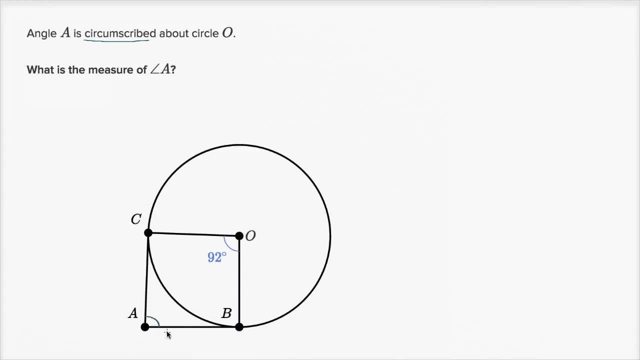 they're segments that would be part of tangent lines. So if we were to continue, so, for example, that right over there that line is tangent to the circle- And let me see if I could so- and this line is also tangent to the circle. 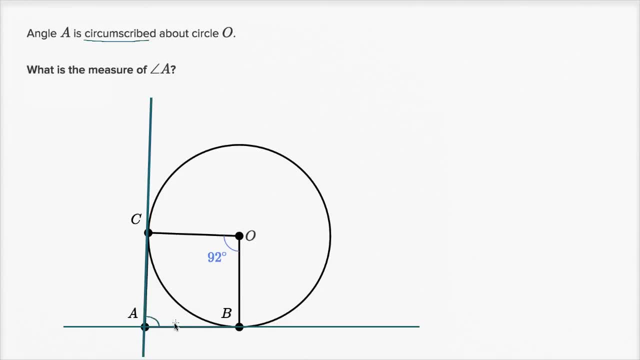 So you see that the sides of angle A are parts of those tangents And points B and point C are where those tangents actually sit on the circle. So, given all of that, they're asking us: what is the measure of angle A? 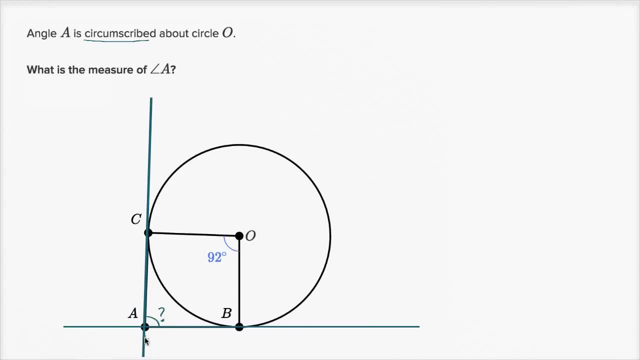 So we're trying to figure this out right here And I encourage you to pause the video and figure it out on your own. So the key insight here- and there's multiple ways that you could approach this- is to realize that a radius is going to be. 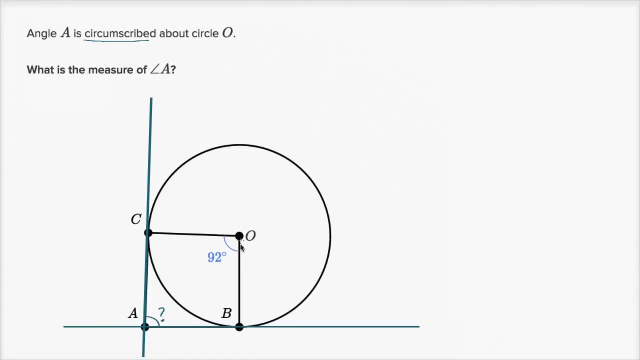 perpendicular to a tangent Or a radius that intersects a tangent is going to be perpendicular to it, So let me label this. So this is going to be a right angle And this is going to be a right angle And any quadrilateral, the sum of the angles. 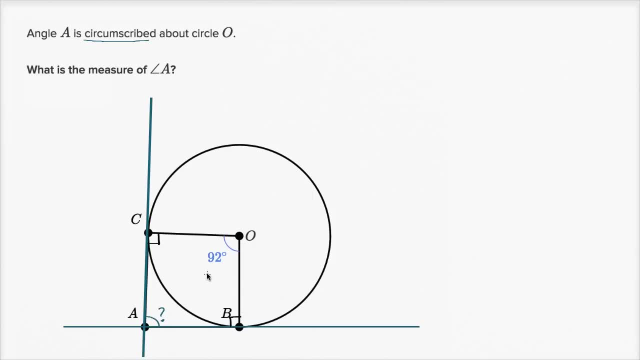 are going to add up to 360 degrees. And if you wonder where that comes from, well, you could divide a quadrilateral into two triangles where the sum of all the interior angles of a triangle are 180, and since you have two of them, 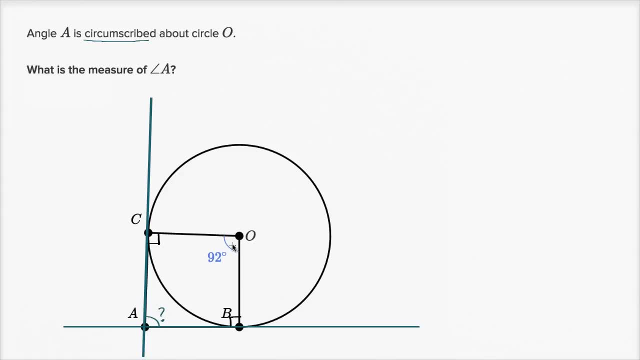 360, 360 degrees. So this 92 plus 90 plus 90 plus question mark is going to be equal to 360 degrees. So let me write that down: 92 plus 90 plus 90, so plus 180,. 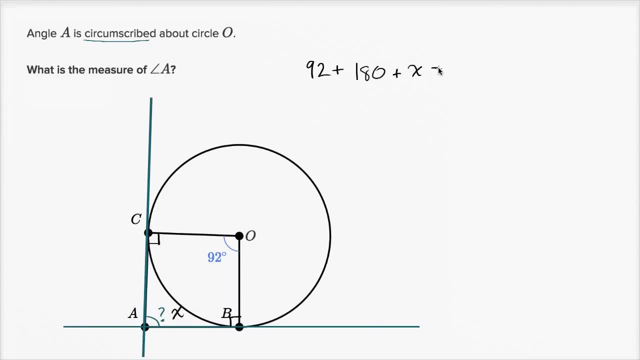 plus let's just call this x, x degrees plus x, They all have to add up to be 360 degrees. So let's see we could subtract 180, 180 from both sides, and so if we do that, 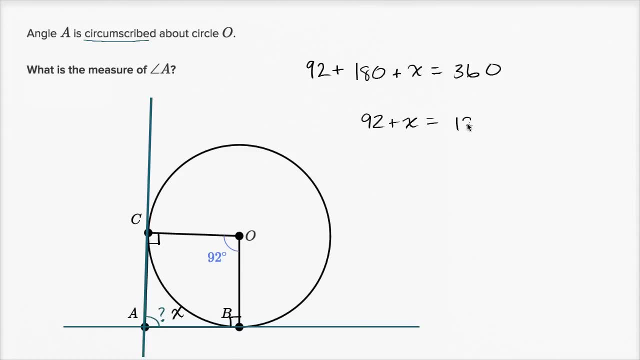 we would have: 92 plus x is equal to 180. And if we subtract 92 from both sides we get x is equal to. let's see, 180 minus 90 would be 90, and then we're just going to subtract two more. 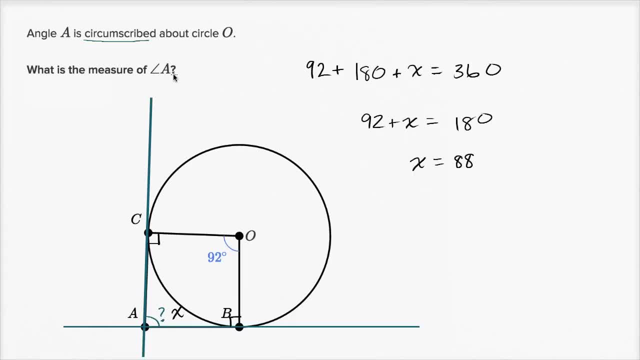 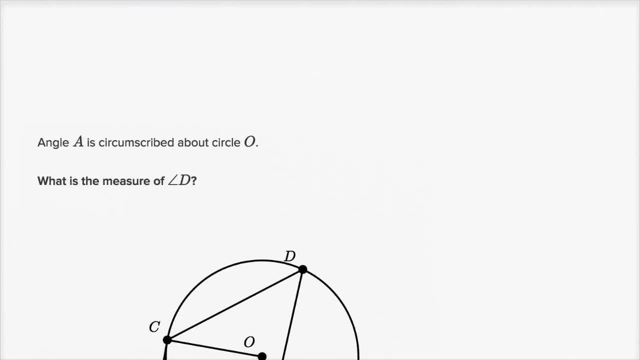 so it's going to be. x is equal to 88. So the measure of angle A is 88 degrees. Now let's do one more of these. These are surprisingly fun, all right. So it says angle A is circumscribed about circle O. 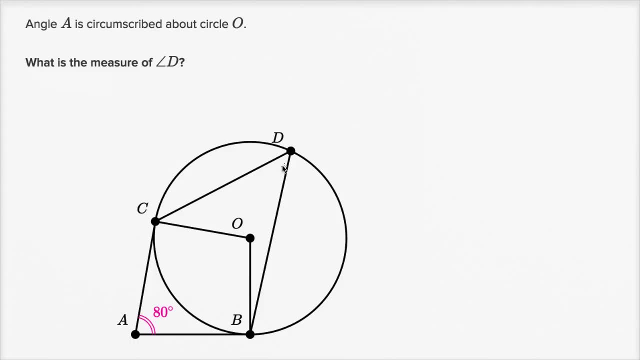 We've seen that before in the last question and they said: what is the measure of angle D? So we want to find, we want to find- let me make sure I'm on the right layer- We want to find the measure of that angle. 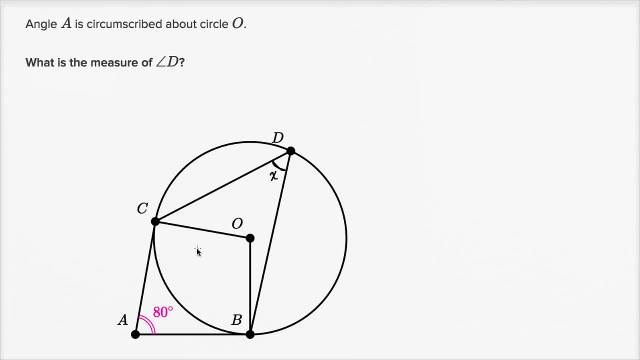 and let's call that, let's call that x again. So what can we figure out? Well, just like in the last question, we have a quadrilateral here, quadrilateral A, B O C, and we know two of the angles. 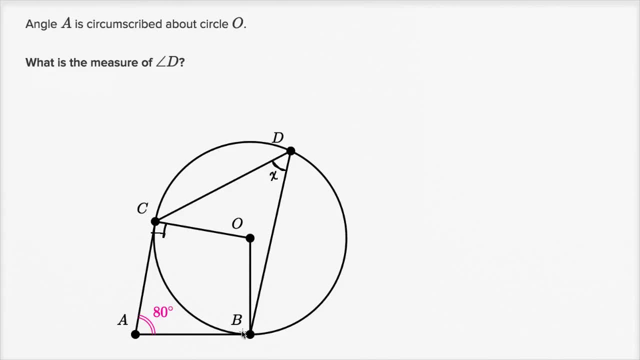 We know this is going to be a right angle. We have a radius intersecting with a tangent Or part of a tangent. I guess you could say, And then this would be a right angle. And so, by the same logic as we saw in the last question, 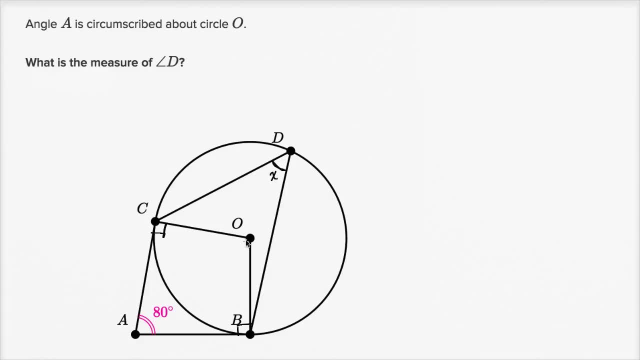 this angle plus this angle, plus this angle plus this central angle are going to add up to 360 degrees. So let's call the measure of this central angle, let's call that y over there. So we have y plus 80 degrees, or we'll just assume everything's in degrees. 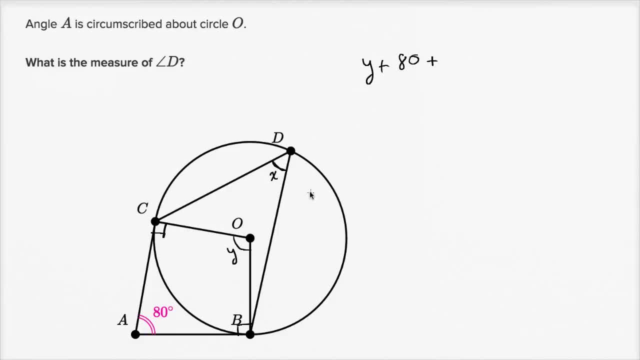 So y plus 80 plus 90 plus 90.. So I could say, plus another 180 is going to be equal to 360 degrees sum of the interior angles of a quadrilateral. And so let's see you have, we could have. y plus 80 is equal to 180. 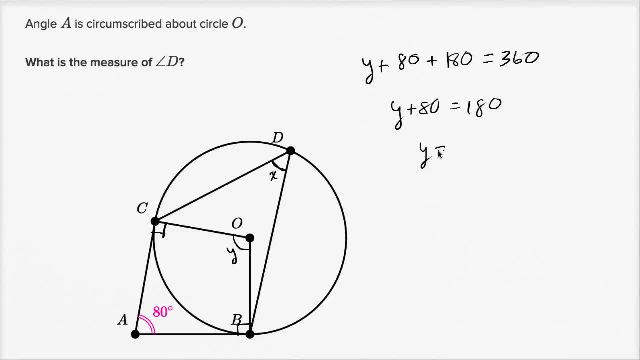 If I just subtract 180 from both sides- I'm gonna subtract 80 from both sides- we get y is equal to 100. Or the measure of this is 100, the measure of this interior angle right over here is 100 degrees. 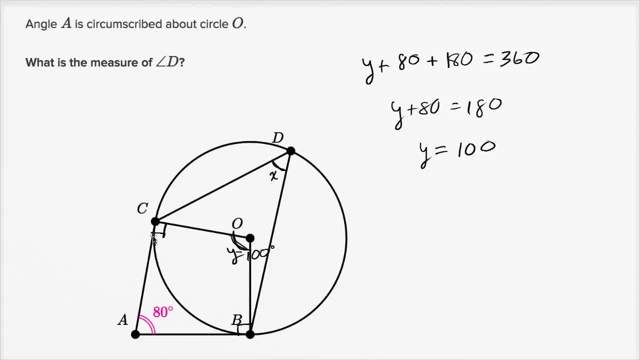 which also tells us that the measure of this arc- because that interior angle intercepts arc CB right over here- that tells us that the measure of arc CB is also 100 degrees, And so if we're trying to find this angle, the measure of angle D, 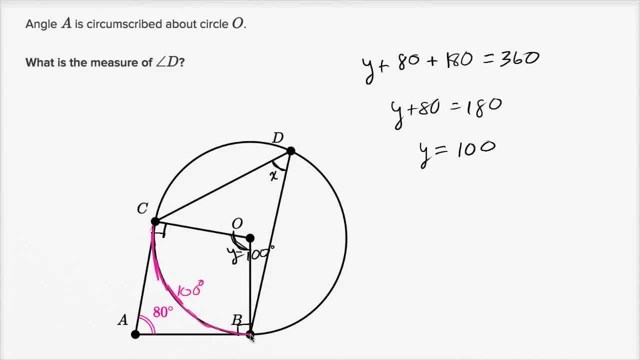 that's an inscribed angle that intercepts the same arc And we've seen in previous videos that that inscribed angle that intercepts an arc is going to have half the arc's measure. So if this is a 100 degree measured arc, 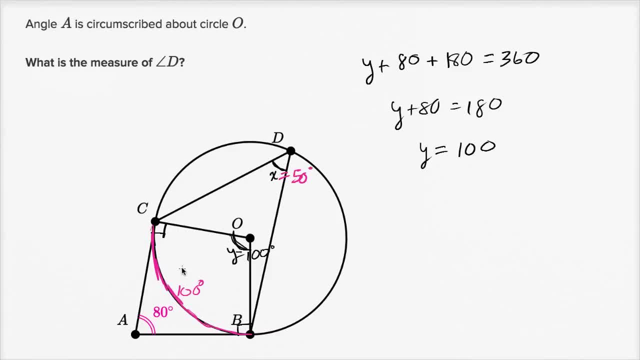 then the measure of this angle right over here is going to be 50 degrees, So the measure of angle D is 50 degrees And we are done.